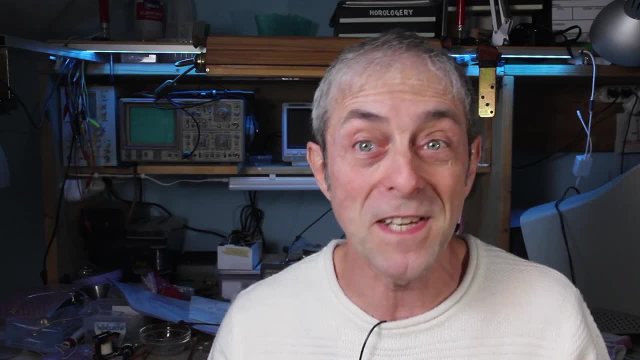 So, for example, if you have a PID control system, you can control it in a very simple way to understand. So, for example, if you have a PID control system, you can control it in a very simple way to understand the whole video if you'd like to learn more about this topic. 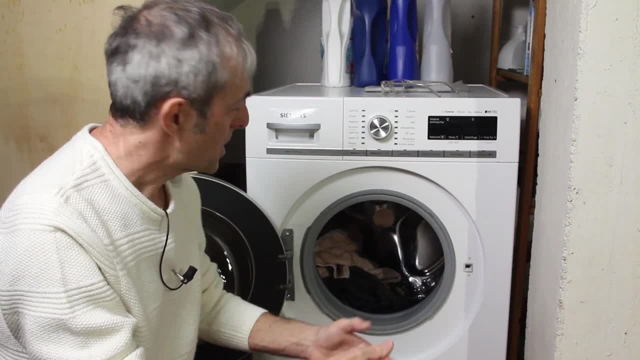 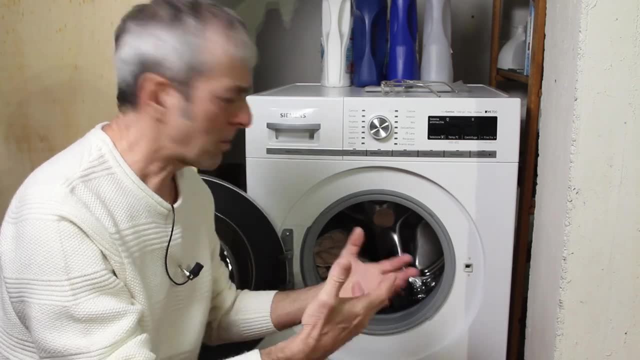 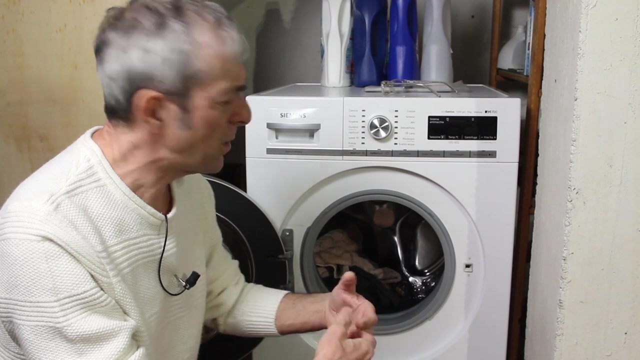 for starters, let's see what the controller system is. so let's take, for example, the motor of a washing machine. its job is to make the drum to spin at a constant speed, so to smash the wet clothes together, to remove the grime from the fibers with the help of 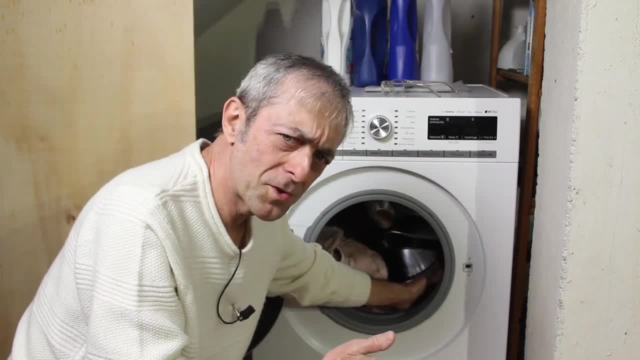 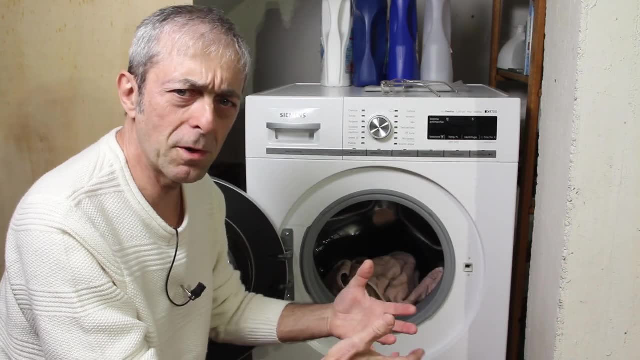 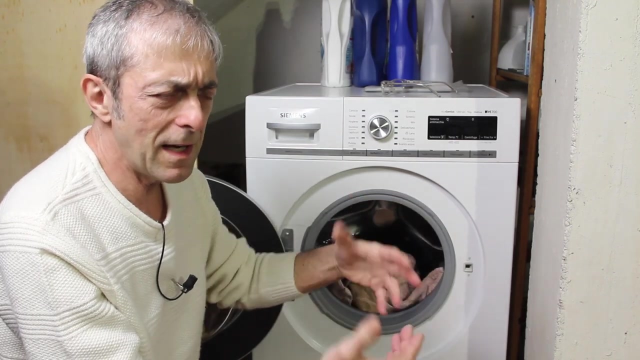 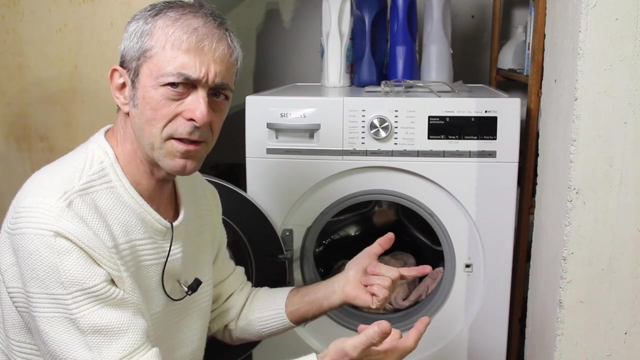 water and soap. however, as the drum moves the laundry toward the top, the laundry falls down and this cause sudden variation in load of the motor for the motor. and this happens even if you have a vertical tab, even though in that case the action is different because it is caused by the interaction between the internal agitator with the external drum. but 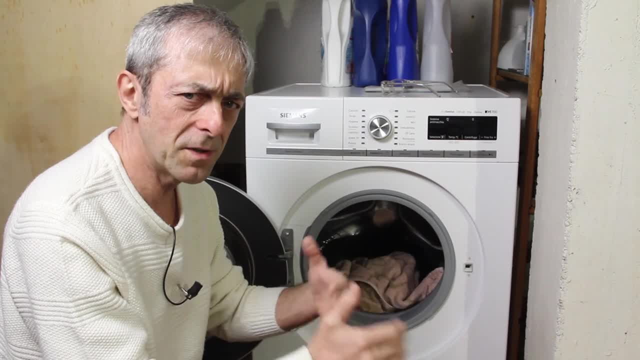 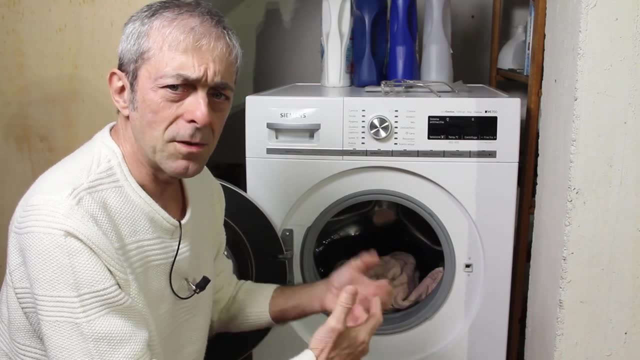 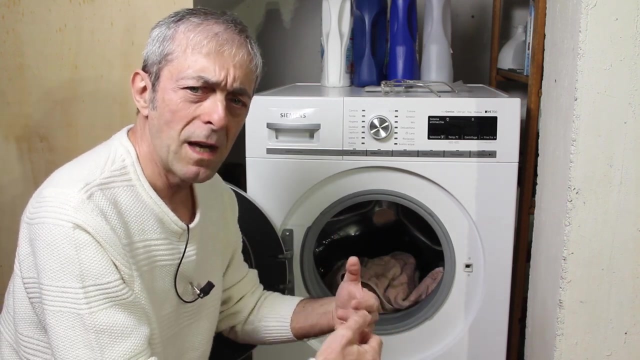 the effect is the same: you have a sudden variation in load for the motor and this jerky load makes the motor to change its speed, degrading the washing action and inducing instability that may lead to increased power consumption and a poor, finer result. so what we can do to prevent all this? 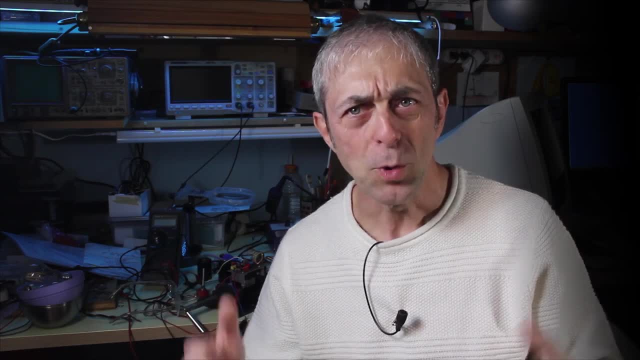 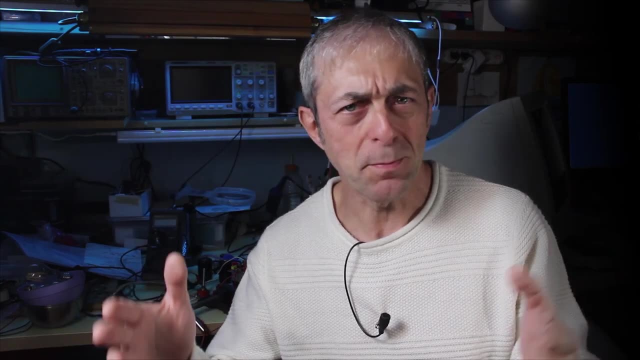 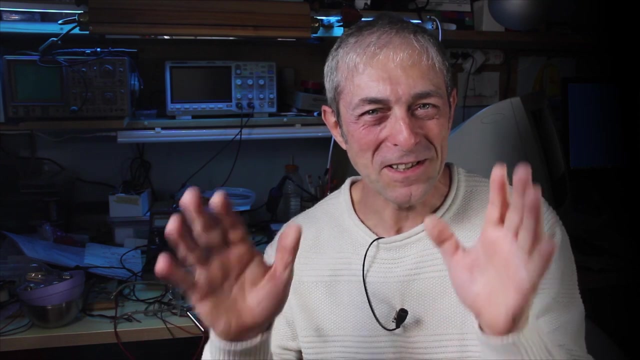 well. to contrast this, we can use a pid, which stands for proportional integral. in contract theory, it is summarized by this formula: ah, that's scary. that's it. well, don't worry, i will try to keep it as simple as possible, so even a perfect noob will understand it well. 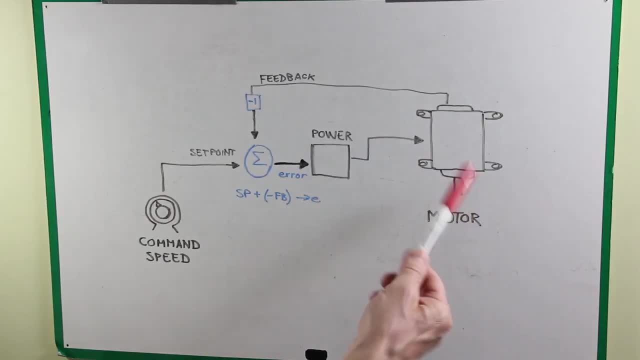 almost, i hope so. to control the speed of the motor we need two elements: the required speed, that is called the set point, and the feedback, that tells us the actual speed of the motor. subtracting these two values or just making the feedback negative and then adding it to. 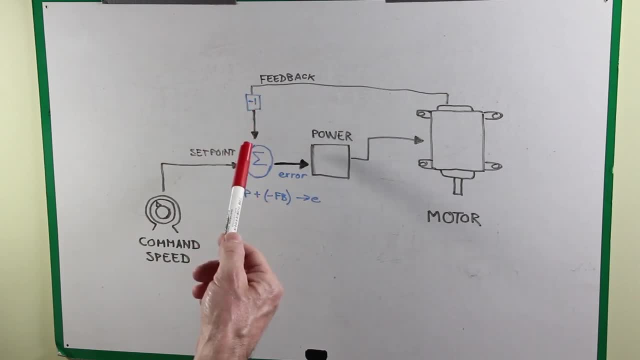 the set point, we get the difference- and that is the error- between the set desired speed and the actual speed, and this error then can be fed into this, the device that provides power to the motor, thus changing the force that the motor exerts to the load and therefore the speed. because of the feedback, the error will be reduced towards zero. 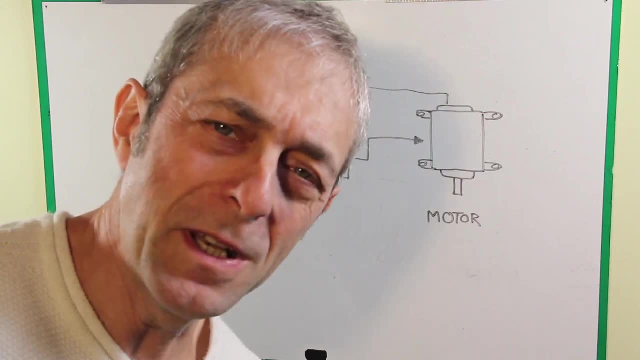 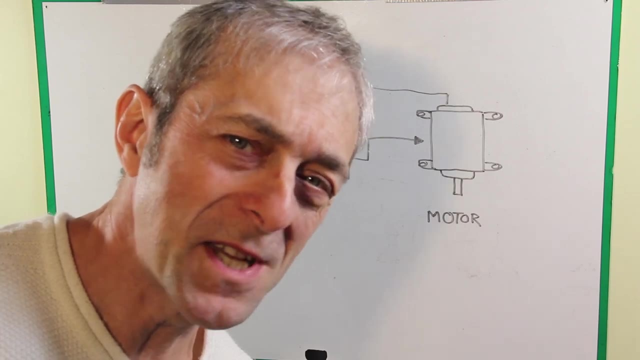 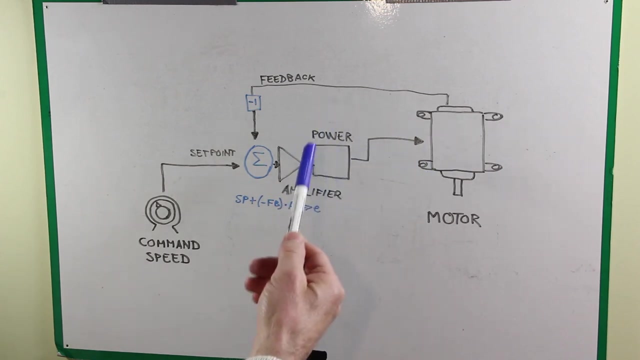 making the motors to spin constantly. well, that would be nice in an ideal world, but because we have losses along the path, we need an amplification to compensate for these losses. however, at this point we may overdrive the device that provides power to the motor, making the motor to suddenly. 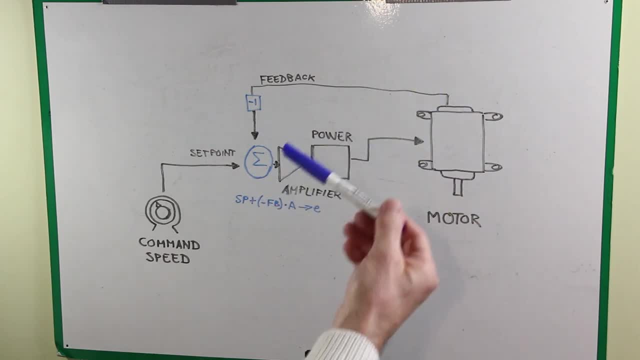 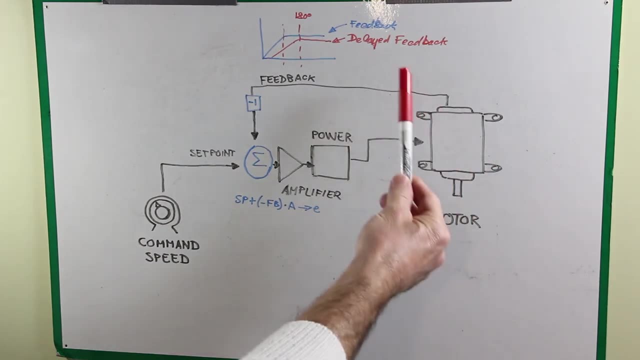 speed up or down at the minimum error too much. also, the mass of the load and of the motor itself introduce a delay that may cause the to feed a signal back which is out of phase, and that is, it reverses and becomes positive. so it adds up with a set point instead of subtracting. 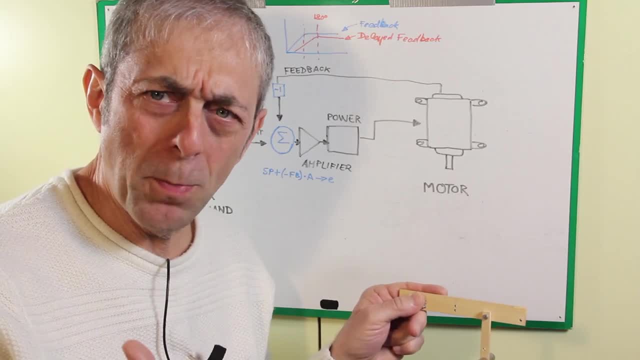 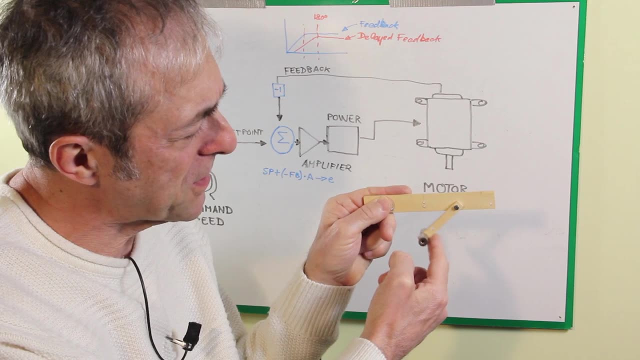 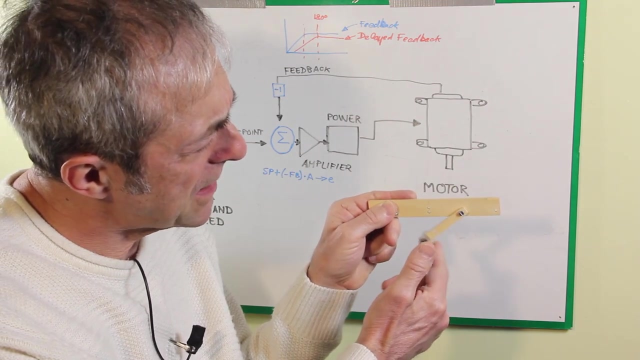 making the whole thing to oscillate. this could be a little bit complex to understand, so let's try to visualize it with the pendulum. pendulum say: if you want to keep the pendulum at a given point out of its rest position, we need to push it, i have to push it. 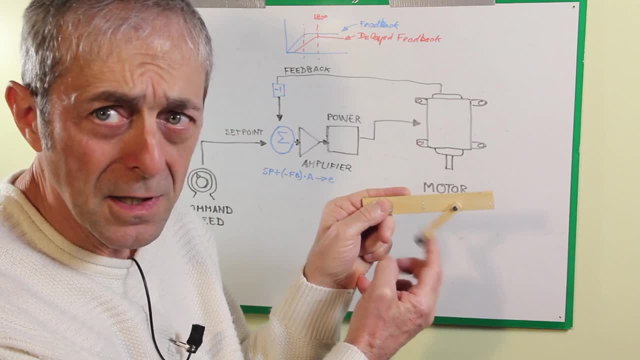 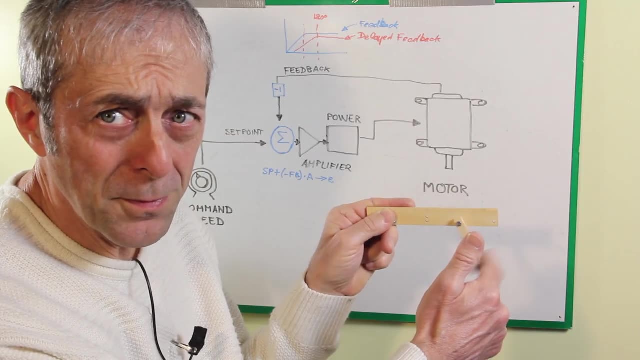 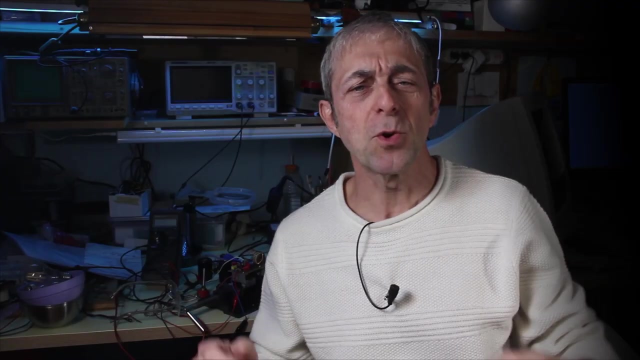 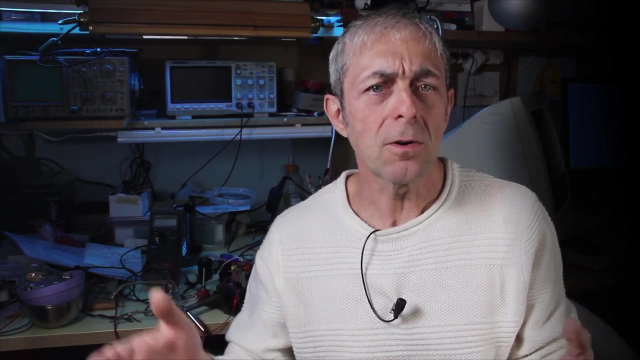 at the right timing and to keep it in position. but if i push too hard or out of phase, the pendulum begins to oscillate instead. so we have the common signal, the set point, the negative feedback assumator and narrow amplifier, and we can translate this into an electronic circuit like this: 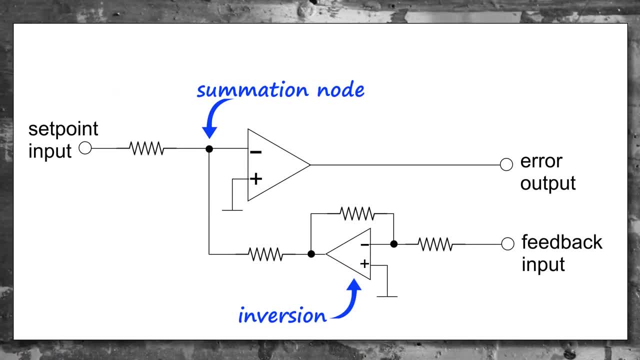 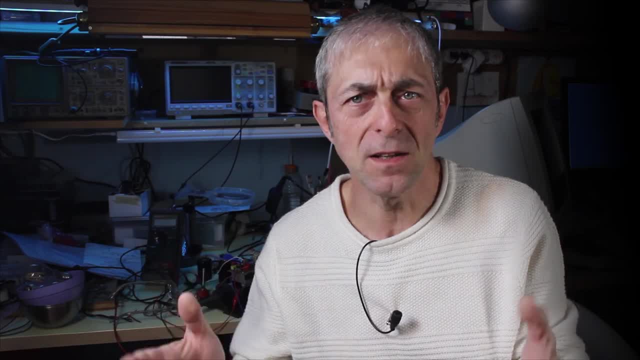 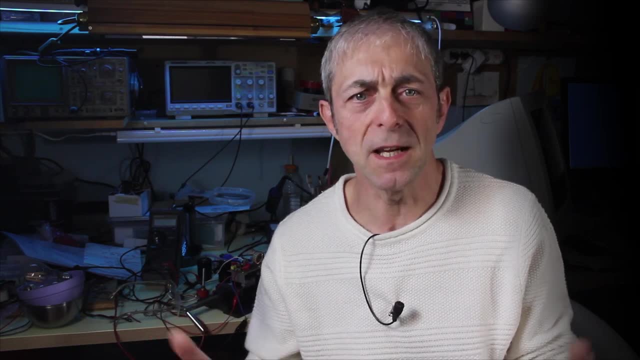 set point. input and the feedback join together into the summation node and then into an operation amplifier that goes to the error output. as we've seen, i cannot amplify the error too much because i run the race to make the whole thing in stable. go figure, an oscillation in a washing machine soon it would make the machine to jump all around the. 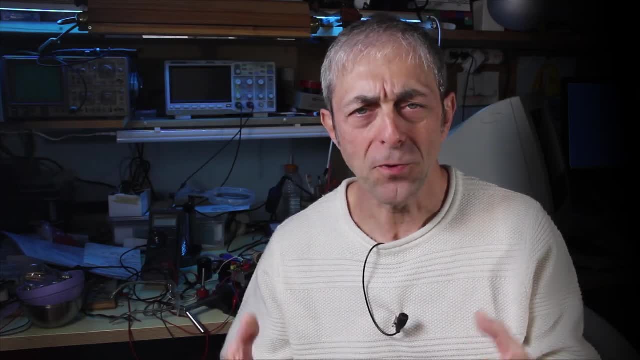 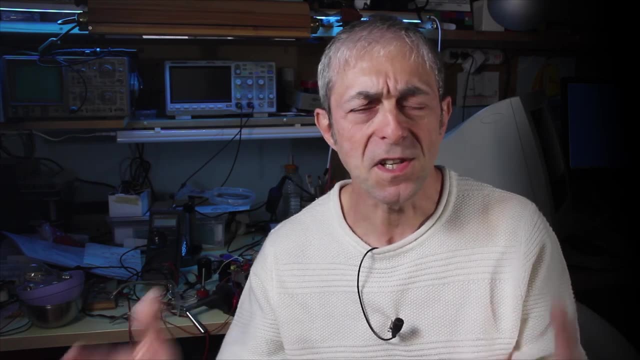 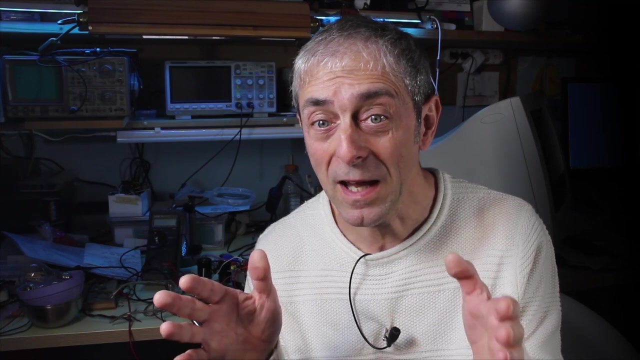 room, though, if we keep the amplification from being too large, at best we will have a constant error, which means the motor will never reach the desired speed. but what if we continuously add the error over time? in that case we can have the effect as a huge amplification, but delayed. 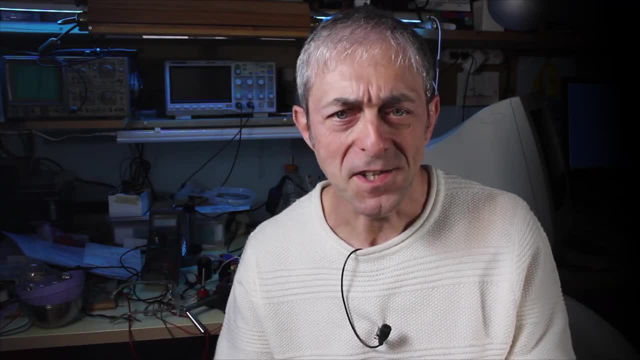 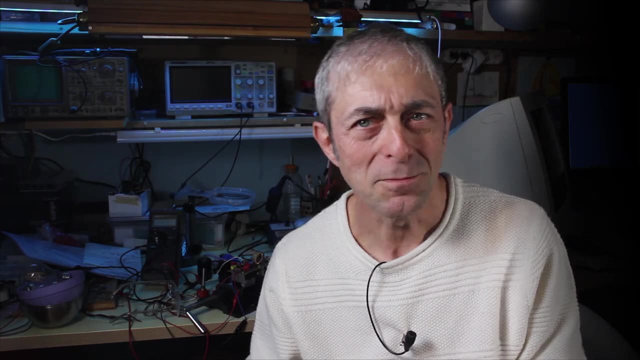 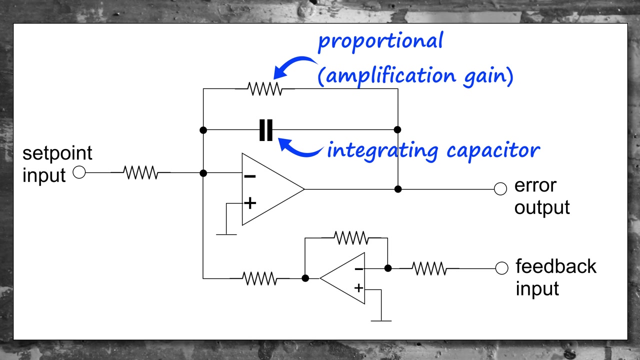 in time. this is what an integrator does. so let's add an integrator to our electronic model, which is now. it's a pi proportional integral. a resistor that carries back the current, the error, to the summation node, controls the proportionality of the error, in other words of the amplification gain. a capacitor connector between the error output. 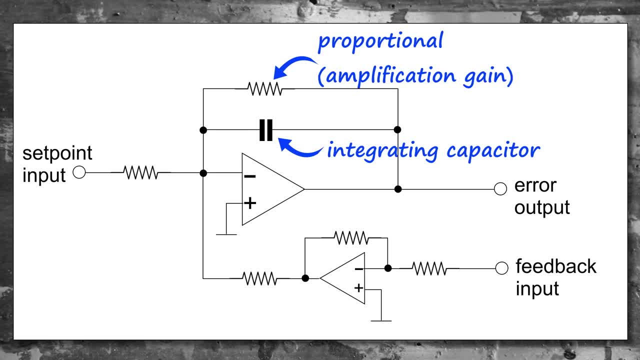 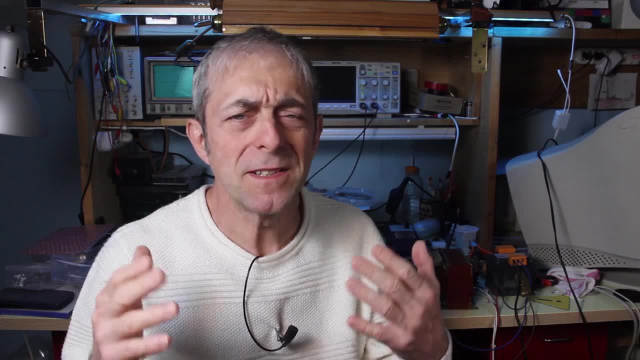 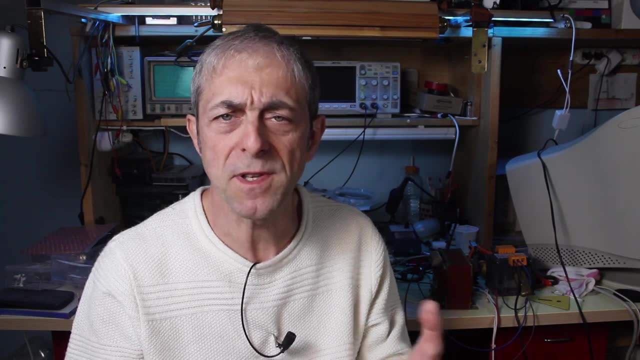 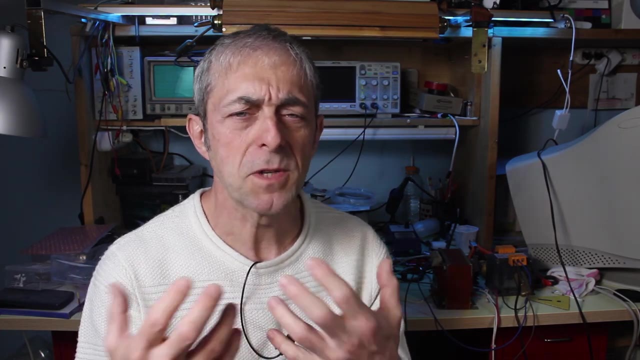 to the summation node operates an integration of the error, while in many commercial applications pi is just enough. what i didn't mention is that an integrator, while is able to reduce the error and to provide more accuracy with stability, it also introduce some kind of sluggish response. We can make the response more aggressive. 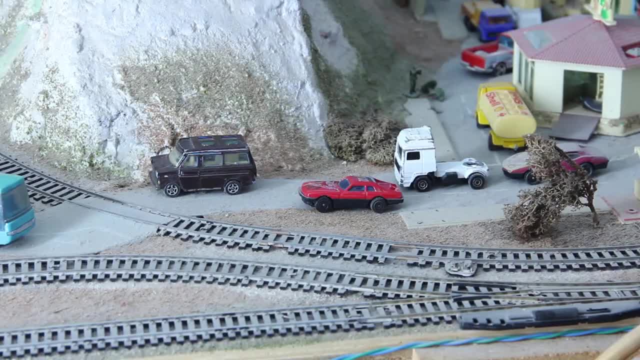 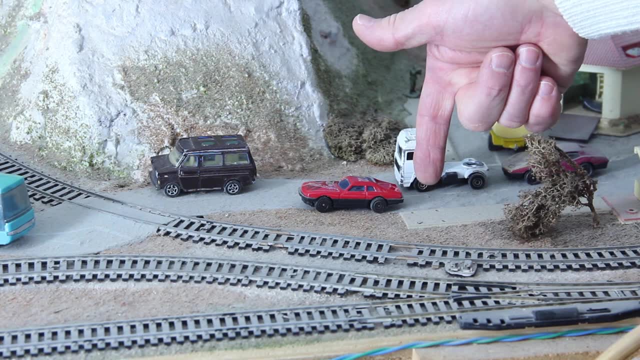 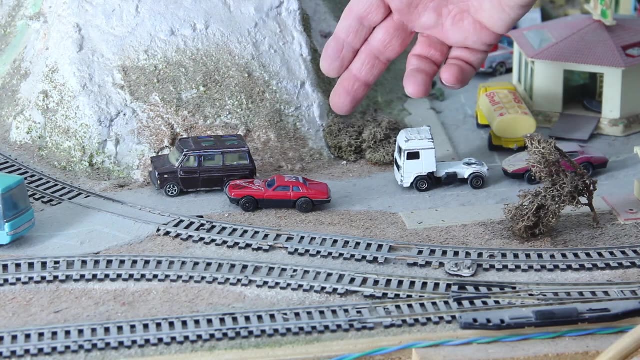 but this will lead to some kind of overshoot. To imagine this, think at when you're driving your car. If you are a bit too aggressive with the gas pedal, the car would overshoot the intended speed and you soon need to release the gas pedal a bit after you realize the speed went too far. 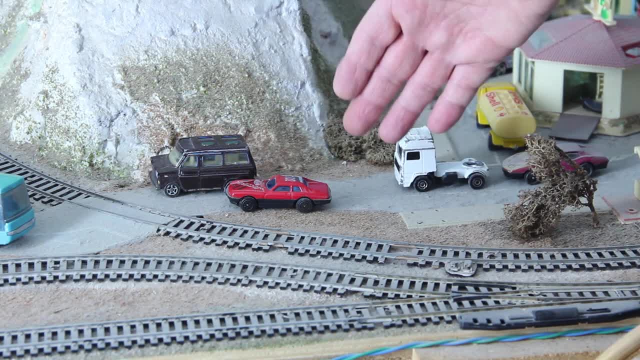 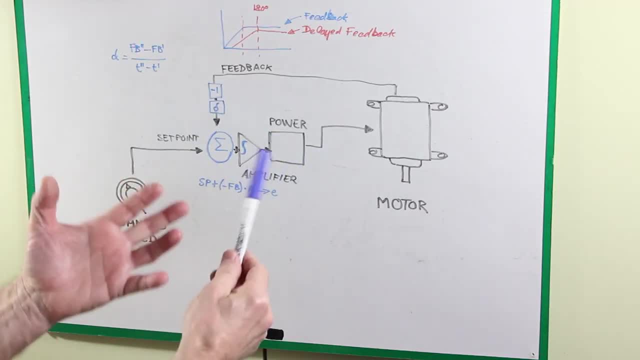 And you can avoid this by predicting what would be the speed of the car. so refrain to push too hard your foot. Similarly, we can add something that works as a predictor of the future trend of the motor speed, and this can be done with a derivative. 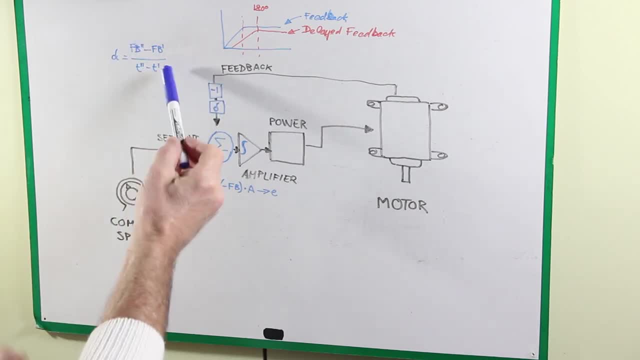 because it provides the difference between the speed now and what it was just a moment before. and this can give you a trend: The more the difference, the more it would be likely, the more the speed would be. In the end, the motor will overshoot. Providing this as a feedback will provide compensation for this trend. 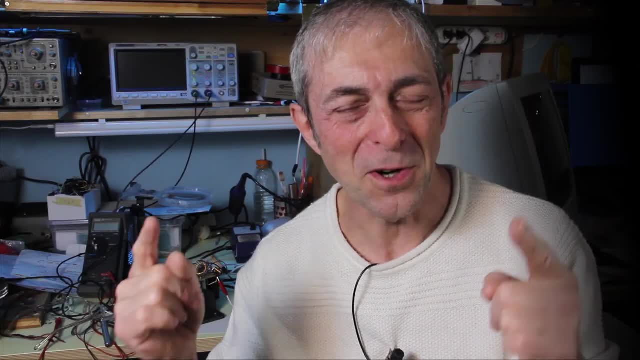 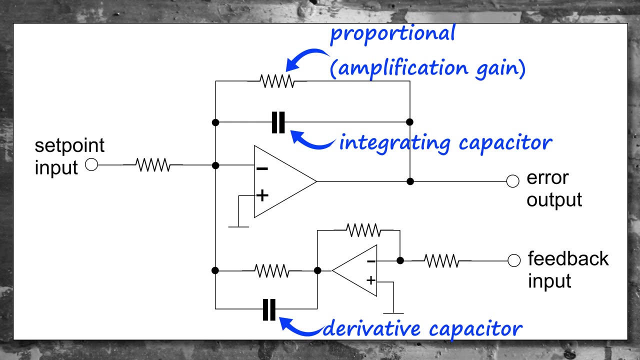 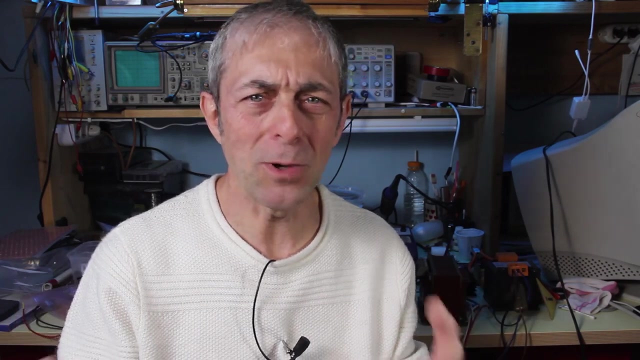 And voila, We have our derivative into our electronic circuit. A capacitor, in parallel with the resistor of the feedback input, operates as a derivative anticipating the variations from the feedback. Well, I hope you've been able to follow me quite easily so far. 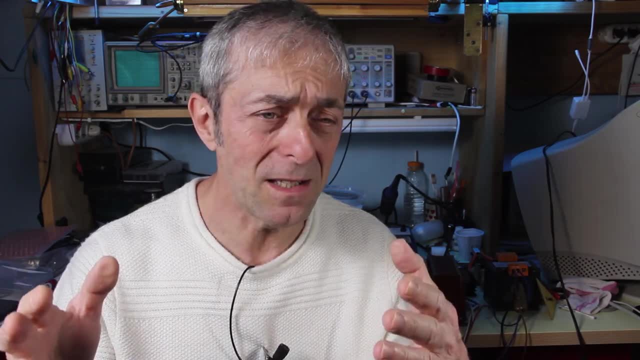 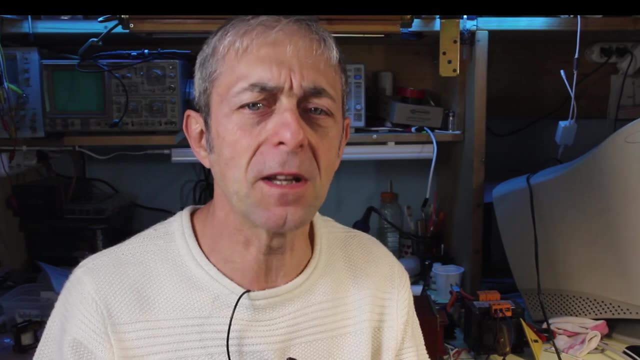 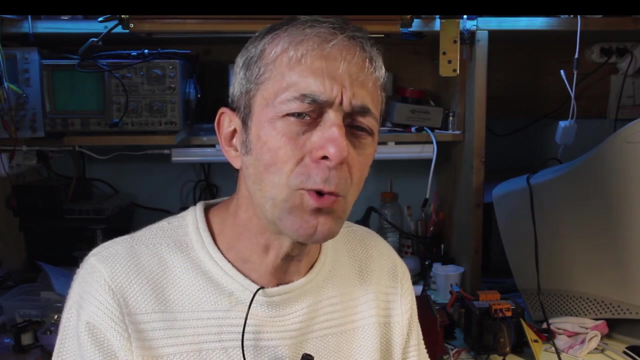 If so, click the like button below. But now let me introduce you into some further considerations. The PID we have seen so far is able to provide a good accuracy and stability. But what if the motor reaches its maximum power and it's not able to cope the acceleration required? 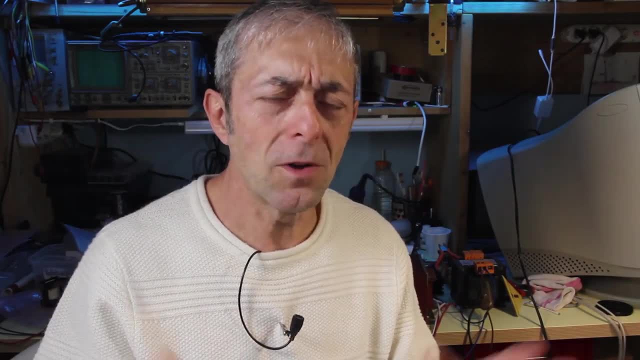 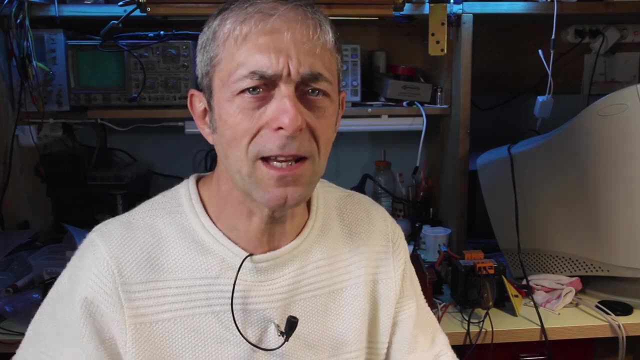 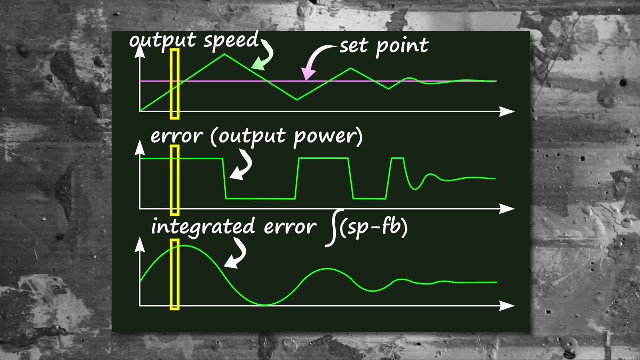 Let's say you push hard the common speed. all of the sudden There is no way the motor can follow this request, so it will just do what it can. However, in the meantime, the error would accumulate over time and when the motor finally reaches the intended speed, 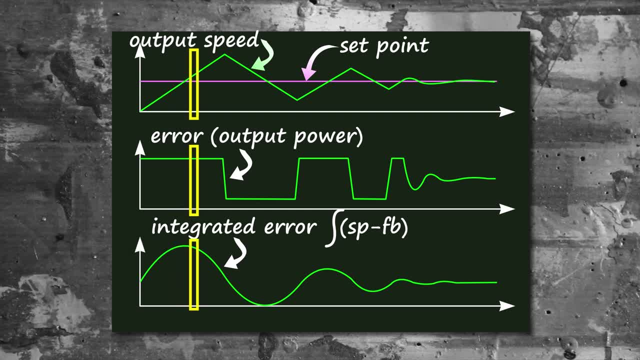 the error would be so large that no derivative compensation would cope with this, causing the motor to continue its run and overshoot spectacularly the intended speed. Because of this, a negative error soon would beat up, making the motor to rapidly decelerate, making again the error to accumulate, and so on. 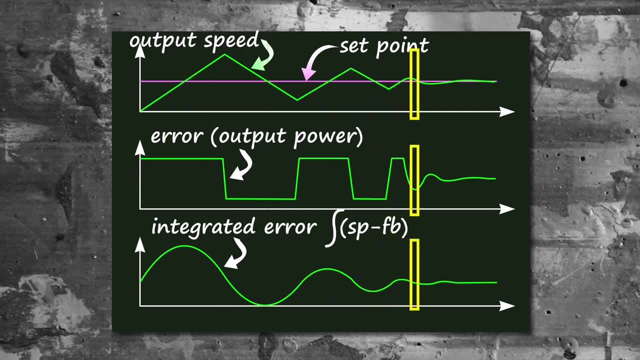 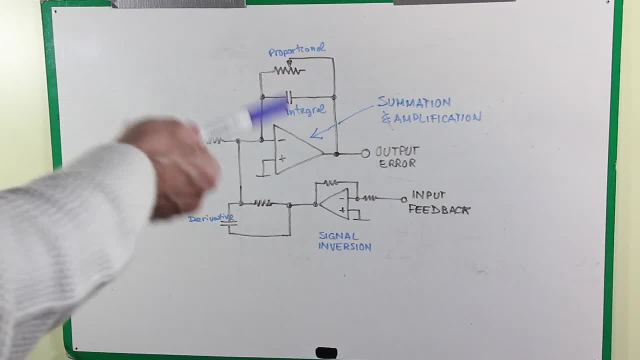 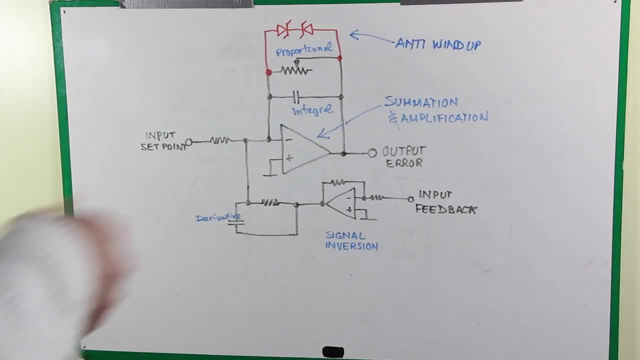 The end result is a damped oscillation made of reliable positive and negative overshoots until the speed finally gets stable. To avoid this problem, we can add a detection when the system got saturated, shutting down the integration. when this happens In our circuit, we can translate this using a couple of zener diodes. 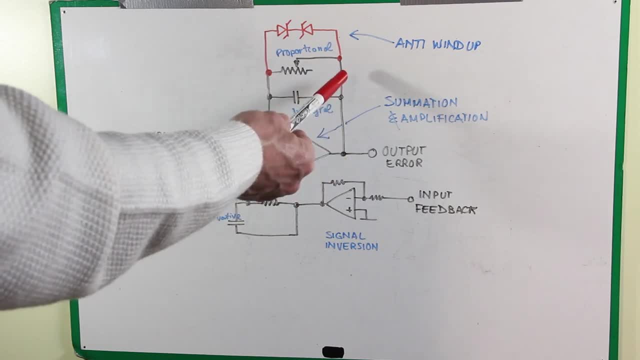 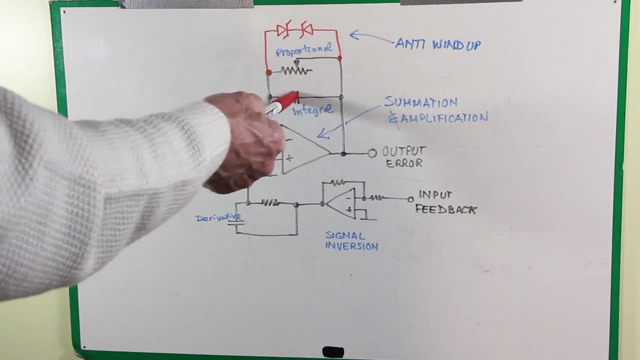 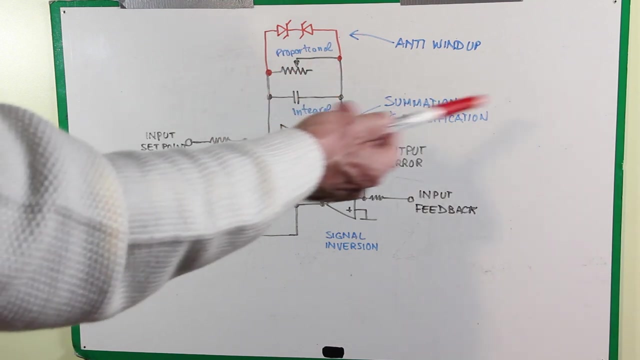 in counter-polarity. As soon as the error amplifier gets closer to the saturation, the zener diode will provide a path that bypasses the capacitor that was used to integrate the error. Of course, this is a proxy of the actual saturation of the power provided to the motor. 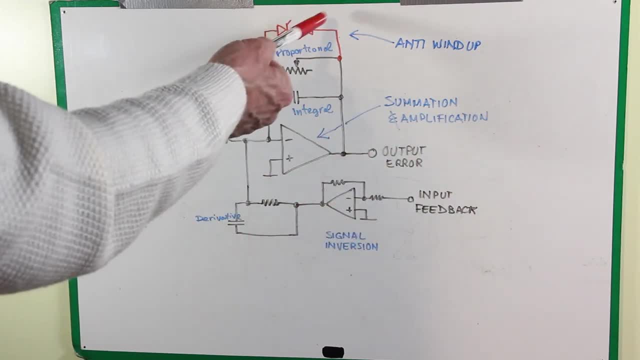 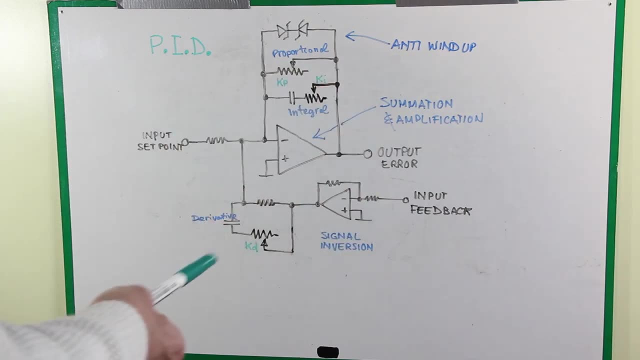 so the value of the zener diodes should be adapted to match the limits of the output power of the motor. Let's make a summary of the final circuit. Here we have this: that works as a summation and amplification, and the sum is made here through these two resistors. 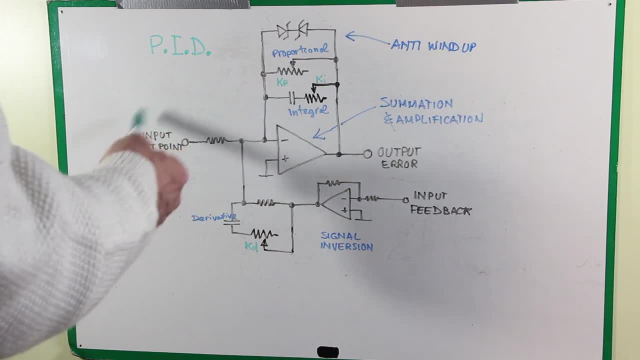 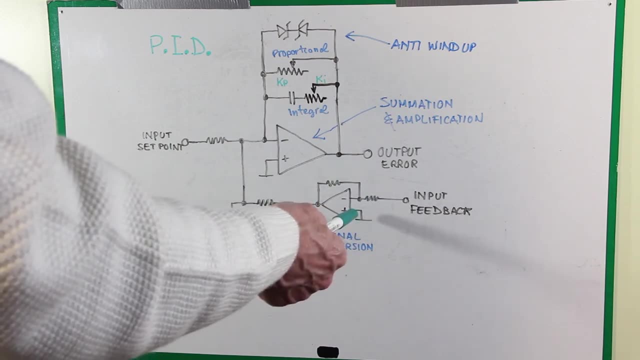 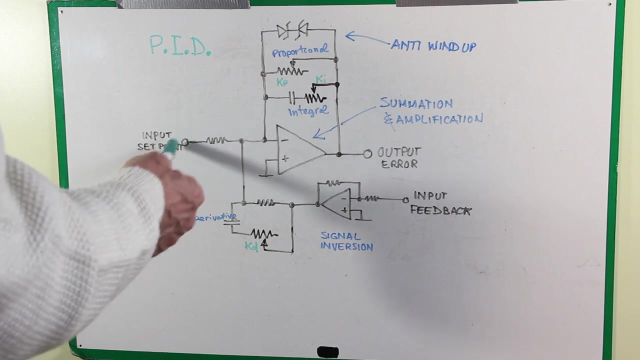 and this from the input set point, the commanded signal, and here from the feedback, and here we have just a signal inversion, so that this signal is subtracted, is actually subtracted from the input signal, so that this signal is subtracted, is actually subtracted from the input signal. 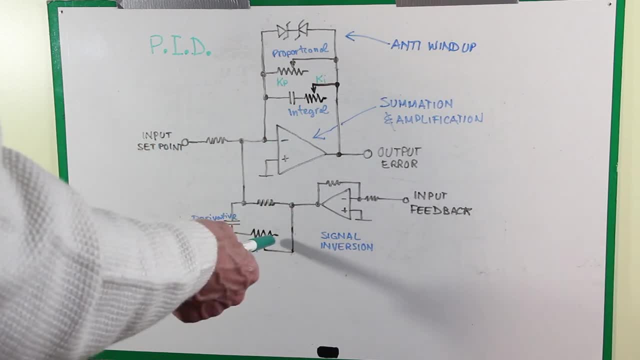 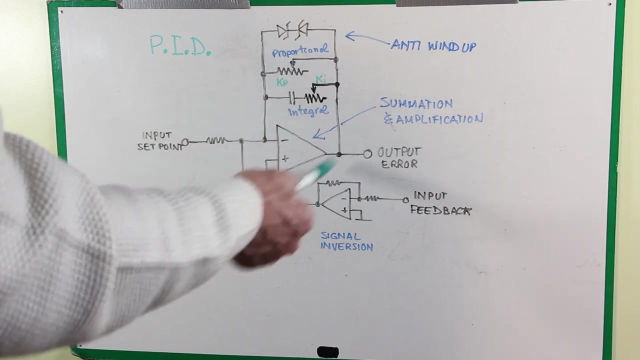 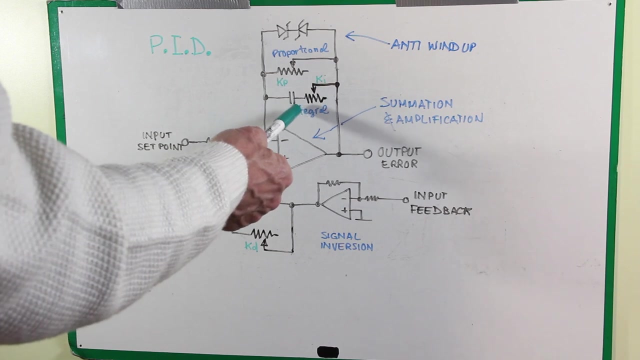 so that this signal is subtracted from the input signal. and here we have the derivative parameter that is adjusted through this potentiometer. and here we have this potentiometer that adjusts the feedback to this operational amplifier, the proportional parameter, and here we have the integral with this capacitor that makes 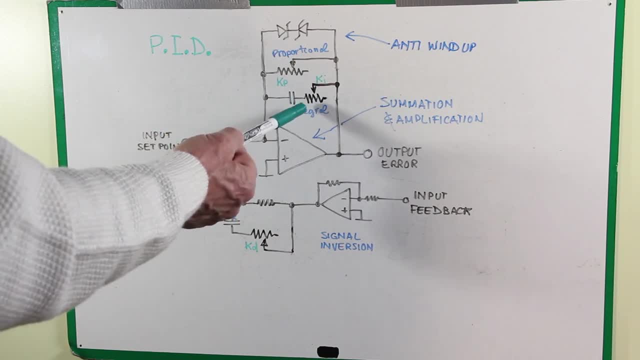 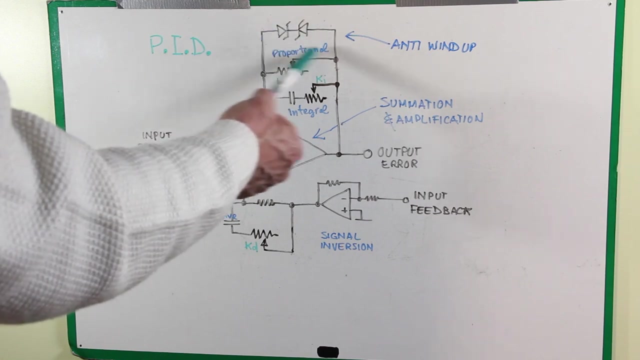 and here we have the integral, with this capacitor that makes that acts as an integrator, and through this potentiometer we can adjust the parameter of the integral. And here we have the two diodes, the two zener diodes that act as anti-wind-up. 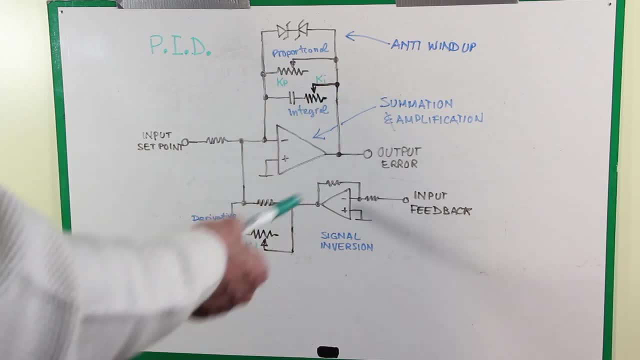 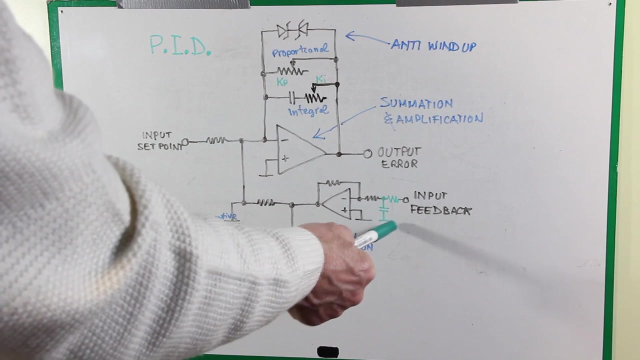 to limit the saturation of the operational amplifier and to prevent the problem we discussed previously. Also a final tip here: to prevent the noise to be amplified through the derivative, we can add just a simple filter to prevent the noise to the high-frequency noise to pass through. 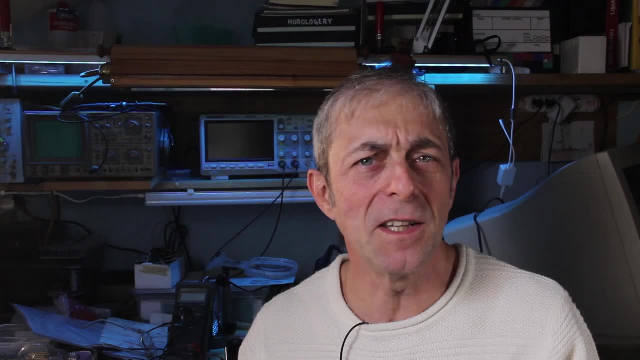 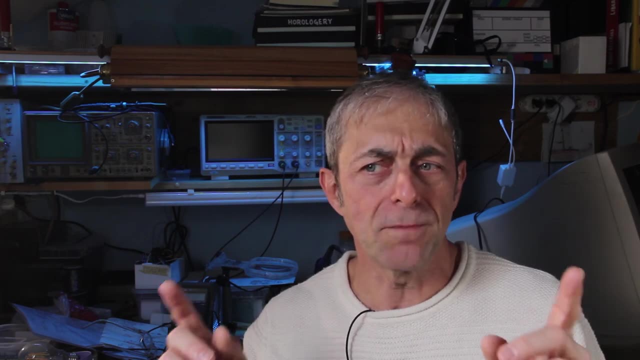 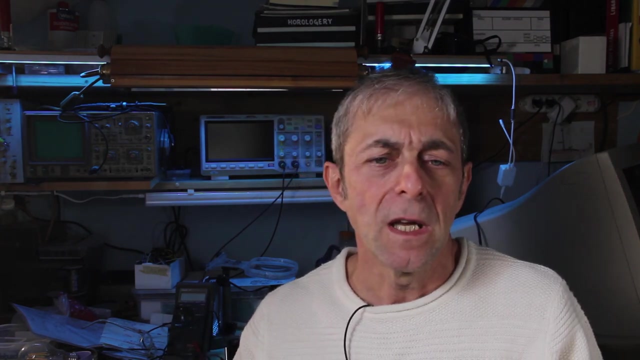 We'll see how to adjust the Kp, Ki and Kd parameters in a future video when I will have a driver for motors ready. Also, check out a previous video where I've showcased driver for a washing machine motor And about this topic I haven't covered all the details. 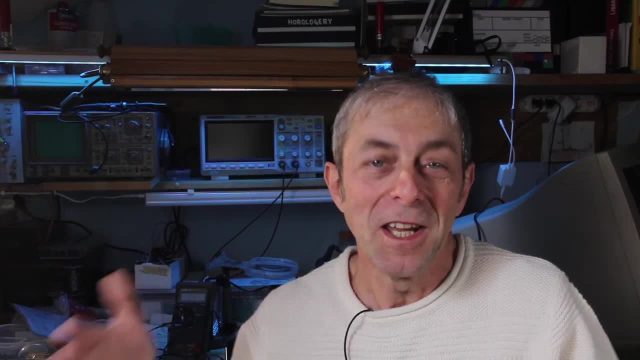 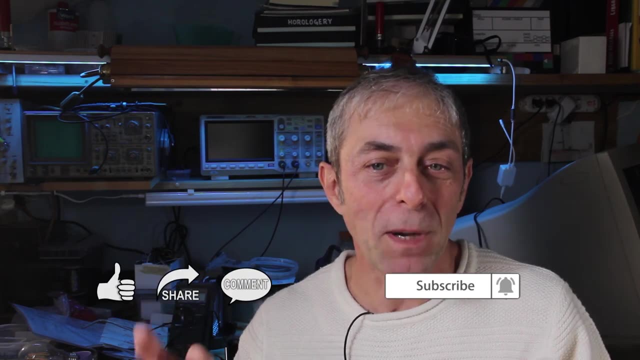 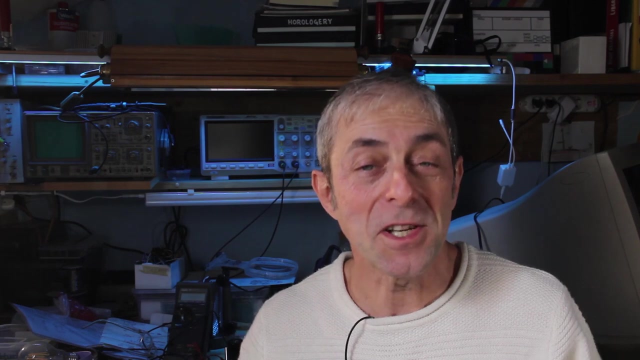 but it would have been beyond the scope of this introductory video. So I hope you enjoyed this video. If so, consider to share and hit the like button, which is a way for me to know I have done a good job. Also, don't forget to leave your comments in the section below. 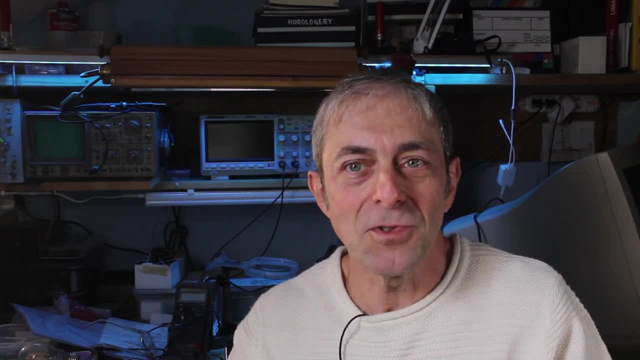 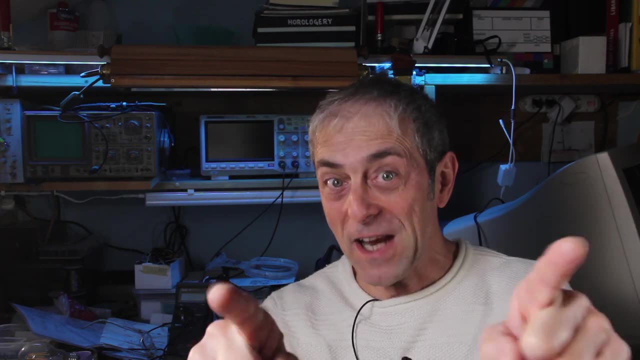 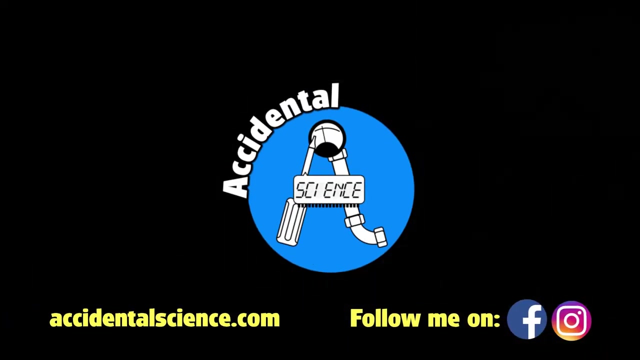 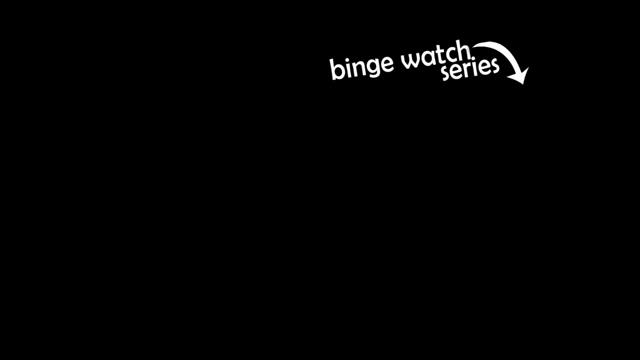 if you have questions or if you just want to say hello. Keep curious and hungry of knowledge. Thanks for watching. See you next time. Bye Captions by GetTranscribedcom.